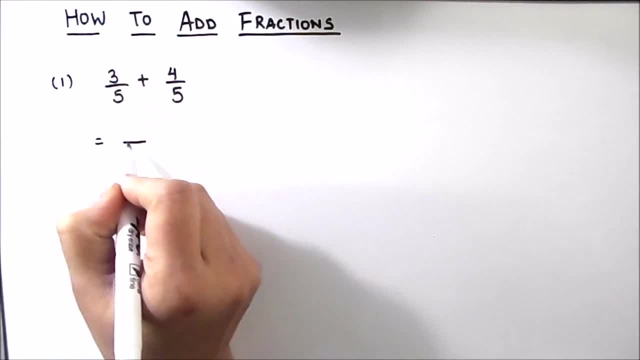 the denominators are same. we can write the two fractions as a single denominator, with the addition of the numerators. So this will be 3 plus 4 divided by 5, which is equal to 7 by 5.. So the final answer. 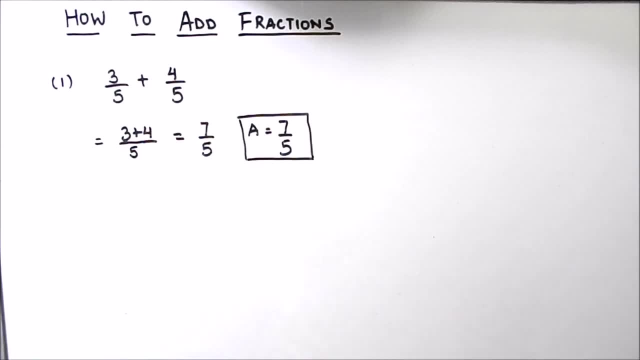 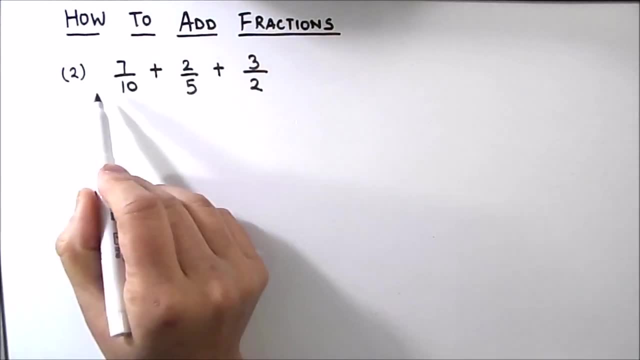 is 7 by 5.. This is the easiest category of fraction addition. Now let us move to our second example. Let's suppose that we have a fraction as 7 by 10 plus 2 by 5 plus 3 by 2 and we need to add: 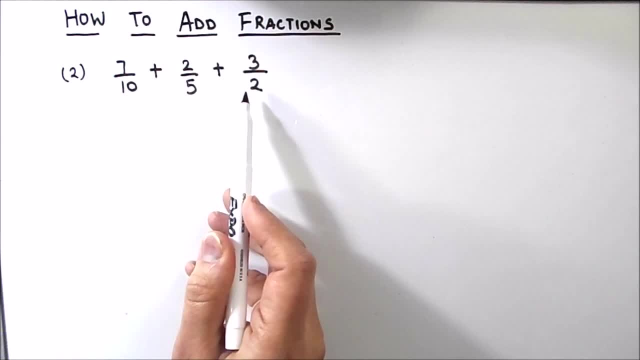 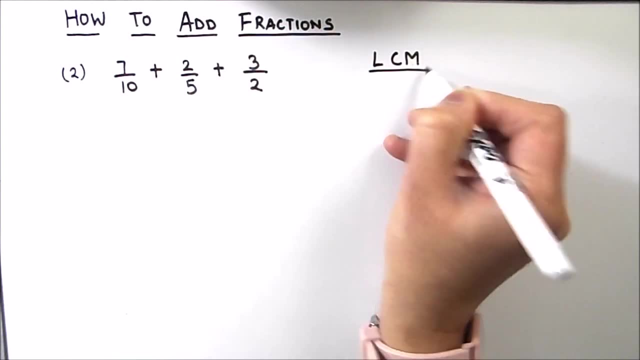 these fractions. The first step in this type of fraction addition is to find the LCM of the denominators. So let's find the LCM of the denominator. LCM is the least common multiple. We divide these three denominators by the prime numbers. So 2 times 5 is 10, 5 is a prime number. 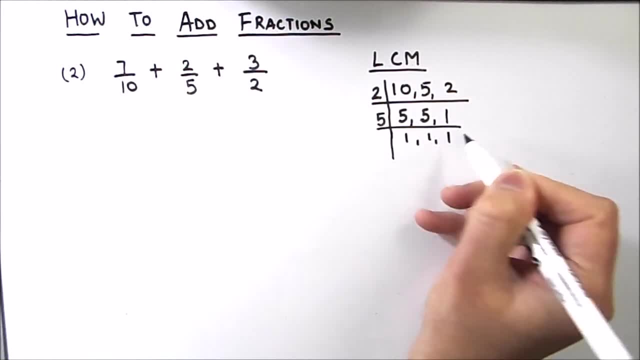 5 times 1 is 5.. LCM will be the product of the two numbers on the left hand side, which is equal to 10.. So our LCM is 10.. Now we will write all these numbers as the denominator as 10.. We already 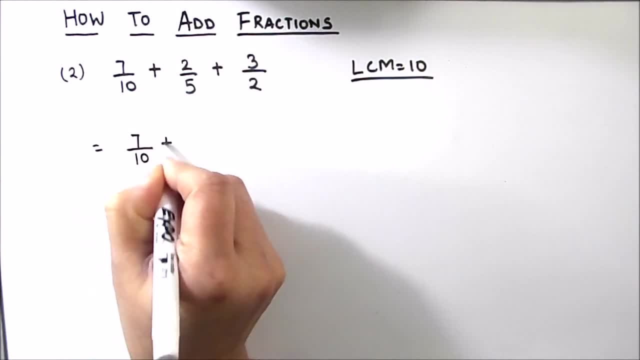 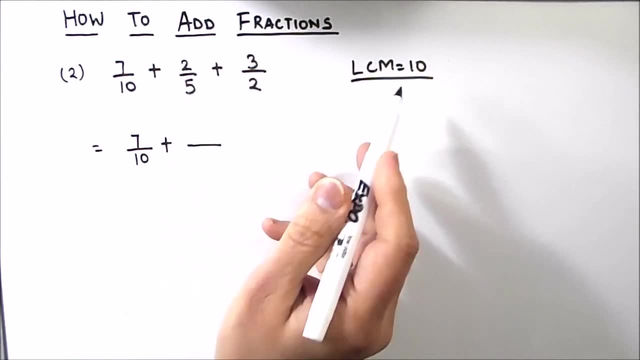 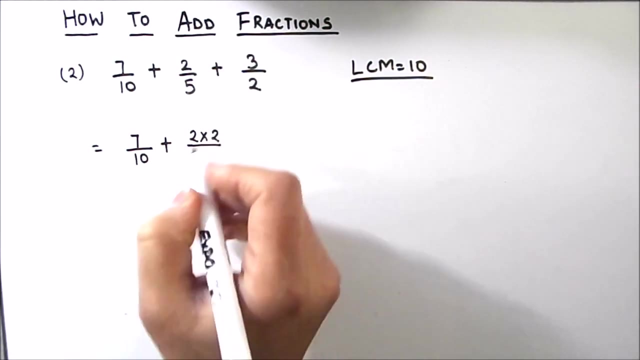 have 10 denominator in our first fraction. So it will be the same 7 by 10.. The second one is denominator 5.. So to make 5 equal to 10, we have to multiply this by 2.. So we will multiply the numerator by 2 and denominator will be equal to 10.. 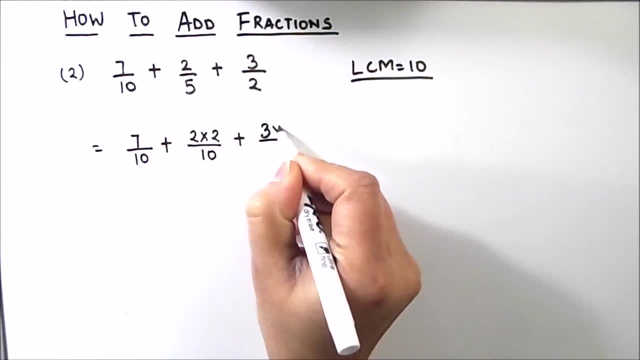 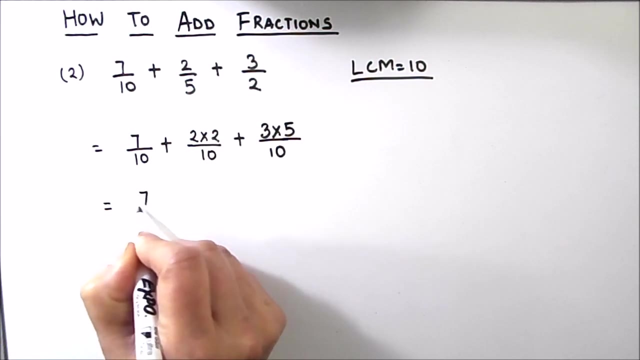 The third one is 3 times. To make this 2 equal to 10, we have to multiply it by 5.. So we will multiply the numerator by 5.. So 3 times 5.. Now 7 by 10 plus 4 by 10. 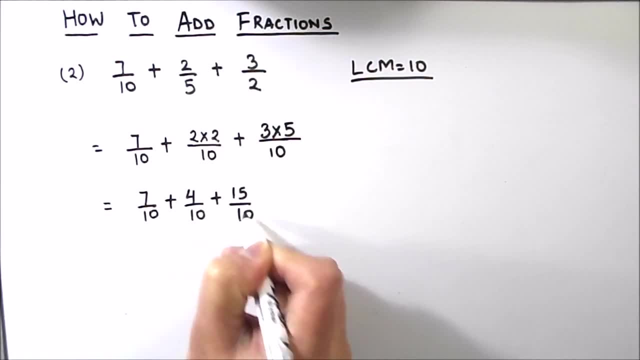 plus 15 by 10.. Now these fractions have the same denominator. We can add all the three fractions directly with the single denominator, So this will be 7 plus 4 plus 15 divided by 10, which is equal to 7 plus 4 is 11, and 11 plus 15 is 26.. So this is 26 by 10.. See that the numbers in 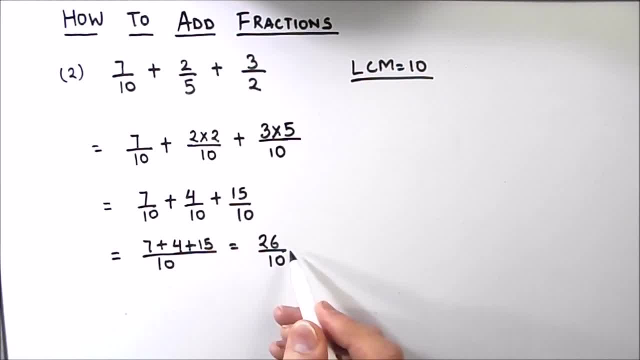 the numerator and denominator. both are even numbers. These can be further reduced by dividing both the numbers by 2 as 2 times 1 and 2 times 3, which is 13 and 2 times 5.. So this is the reduced form of our answer, which is 26 by 10.. So the answer is 13 by 5.. 26 by 10 is also correct, but 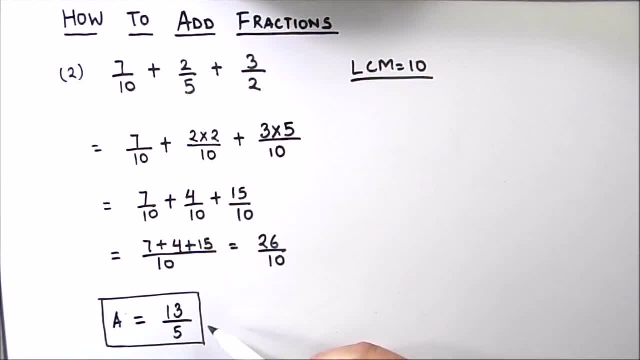 it is a good practice to write fractions always in the reduced form. So the reduced form of 26 by 10 is 13 by 5.. So our final answer is 13 by 5.. So for adding fractions with different denominators, 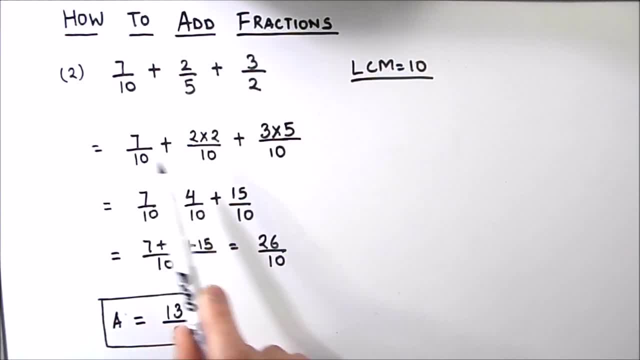 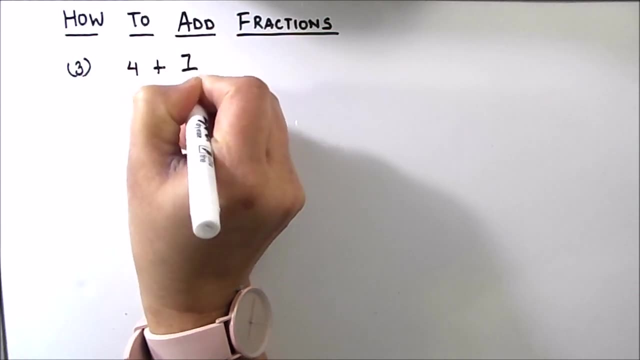 we have to first take the LCM of the denominators, make the denominators of all the fractions the same, and then we can further simplify and add the fractions. Now let's move on to our next example. Our next example is 4 plus 7 by 8.. So, as you see here that 4 plus 7 by 8 is equal to: 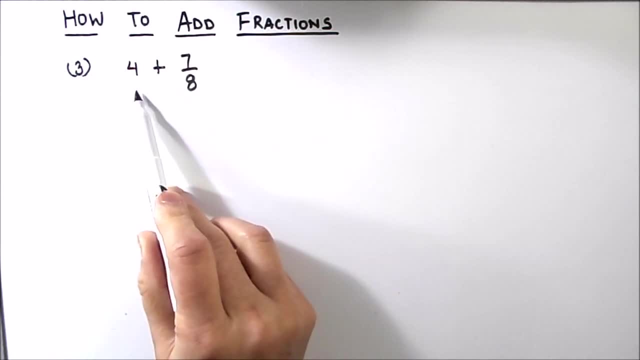 4 is not a fraction here and 7 by 8 is a fraction. So a number, a whole number and a fraction addition. you can see This is one way of seeing this fraction. But we all know that all natural numbers can be written in the form of rational numbers, which is 4 divided by 1.. So 1 is the. 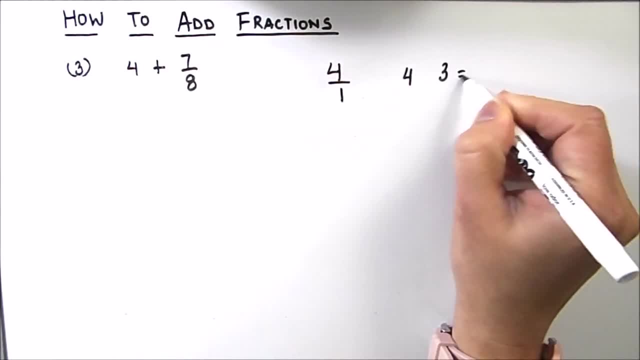 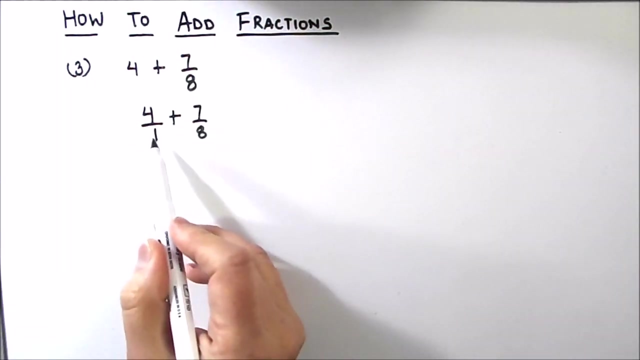 denominator of all the whole numbers, because 3 is equal to 3 by 1.. 5 is equal to 5 by 1.. So normally the practice is not to write the denominator as 1.. All whole numbers consist of the denominator as 1.. We can write this 4 as 4 by 1.. Now we have two fractions adding. 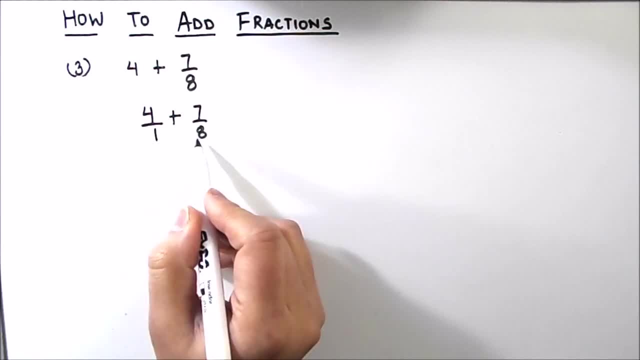 together. Next step is to make these denominators equal. Now, as this is 1 and this is 8, the LCM will be 8.. So 1 times 8 is 8.. So the numerator will be 4 times 8.. And the second fraction will. 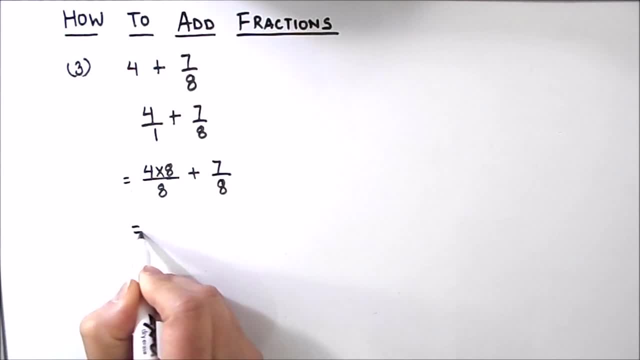 be 7 by 8, because 8 is the LCM. So 4 times 8 is 32.. So this is 32 by 8 plus 7 by 8, which is equal to 32 plus 7 divided by 8, which is equal to 39 by 8.. We see that. 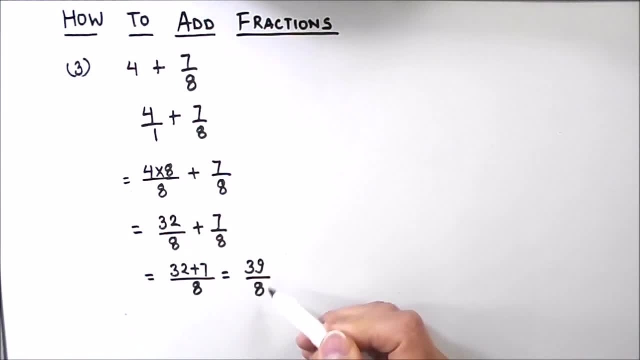 the numerator is an odd number and the denominator is an even number, So we cannot reduce this fraction further. So our final answer will be 39 by 8.. Let's move on to our next example, in which we are adding two mixed fraction. The addition of mixed fraction is same as: 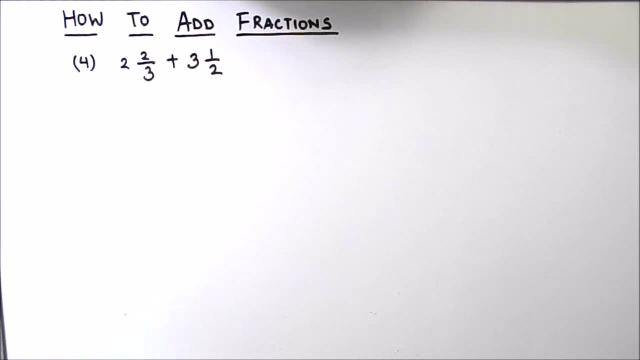 fraction. There will be an extra step, which is the first step, to convert this mixed fraction into a improper fraction. So first we will convert this mixed fraction into improper fraction. So this will be 3 times 2 plus 2 divided by 3 plus 2 times 3 plus 1 divided. 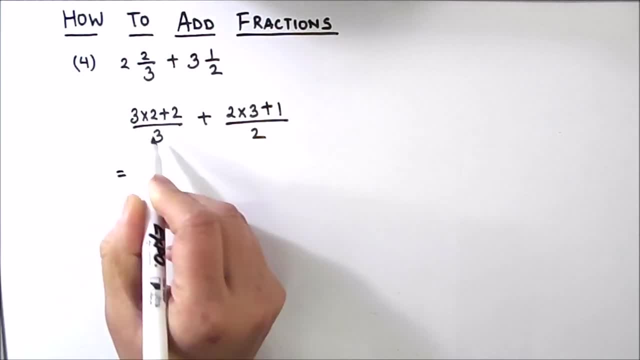 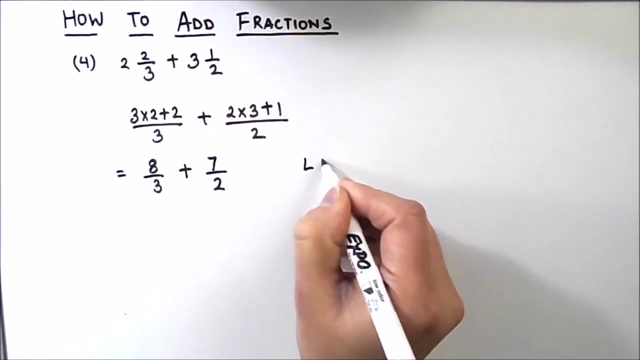 by 2, which is equal to 6 plus 2, is 8.. 8 by 3.. 8 by 6 is equal to 6 plus 1 is 7.. 7 by 2.. The next step is to find the LCM of the denominators. The LCM of the denominators is the 6. Cos. 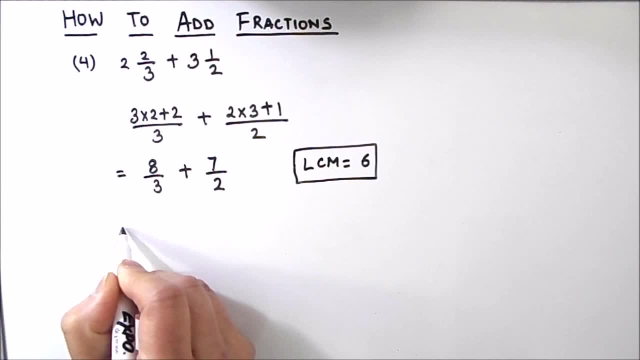 3 times 2 is 6.. Now we will make both the denominators as 6.. So 3 times 2 is 6.. So we will multiply numerator by 2, and in the other fraction we have 2 times 3 is 6.So we will. 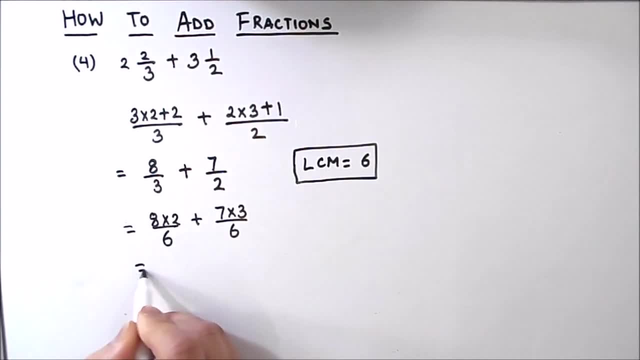 multiply the numerator by 3.. So 8 times 2 is 16.. 16 divided by 6 plus 7 times 3 is 21.. 21 divided by 6.. Now we will add the two fractions, So 16 plus 21 divided by 6, which is equal to 37 by 6.. 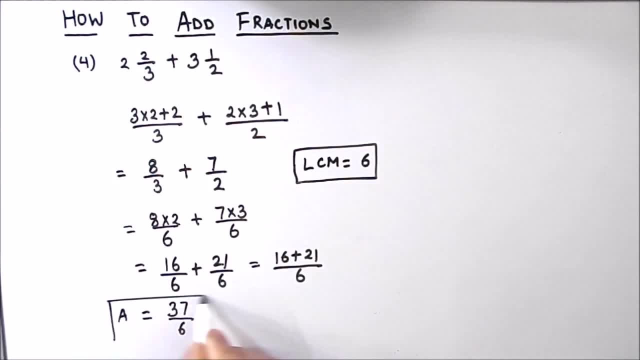 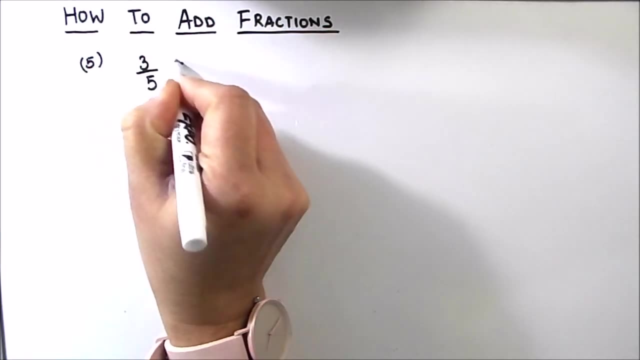 So our final answer is 37 by 6.. Addition of mixed fraction is the same as the fraction, except that we have to first convert these mixed fraction into improper fractions. Now let's move to our final example, which is 3 by 5 plus 2 by 7.. Here too, the first step is to find the LCM.